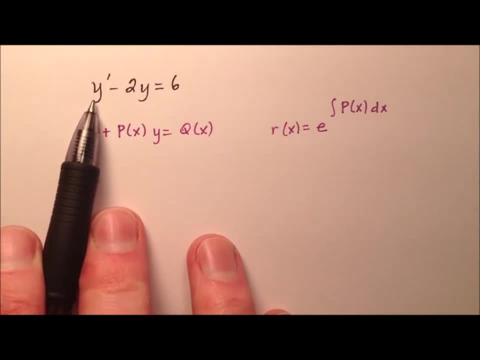 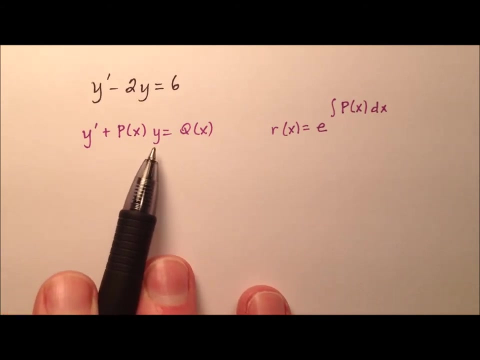 y as a function and one of its derivatives. So we consider this equation first order because the highest derivative we see is the first derivative. Also, we consider this linear because it can be written in the form: y prime plus p of x. y equals q of x. All right, well, p of x and 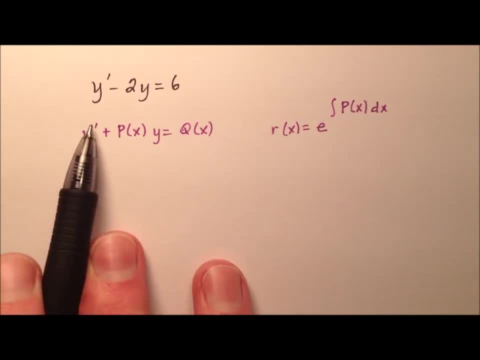 q of x are just functions in x and the y prime notice is by itself. So it looks like the equation that we're given here in the first example is already written in this linear form. So the p of x function is the first derivative and the first derivative is the first derivative. So 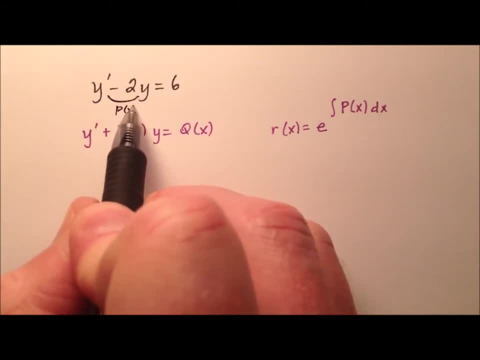 the first derivative is going to be the negative 2, and the 6 right here is going to be our q of x. Okay, well, we've got this kind of expression over here, this r of x. We're going to call this the. 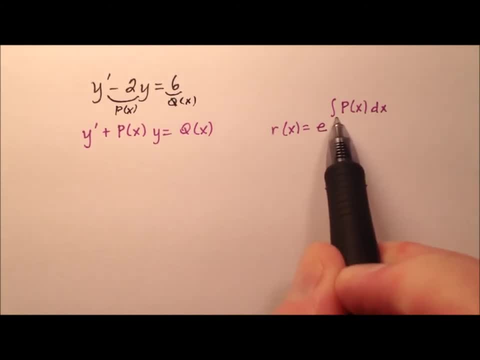 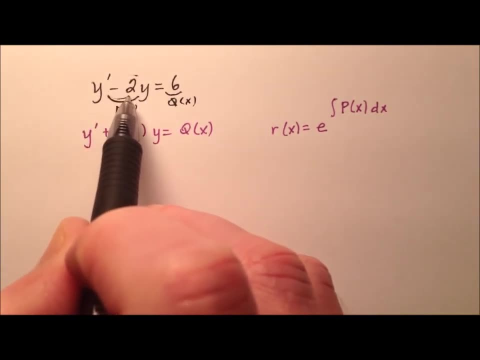 integrating factor and it's going to be e to the power of the integral of p of x, dx. So this p of x function, whatever function in x is with the y, is going to be important because we're going to integrate that and then put it as a power of e. So let's go ahead and do that. So negative 2 was our. 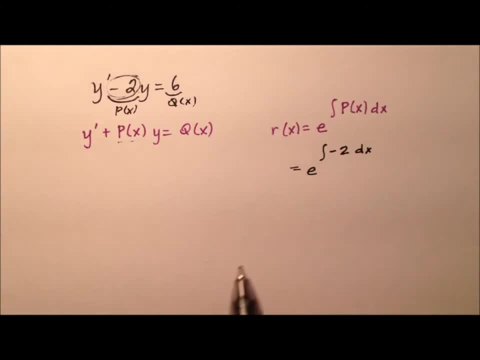 p of x and we're going to integrate that with respect to x. So when I integrate negative 2 with respect to x, I'm just going to get negative 2x. So our integrating factor, this r of x, is going. 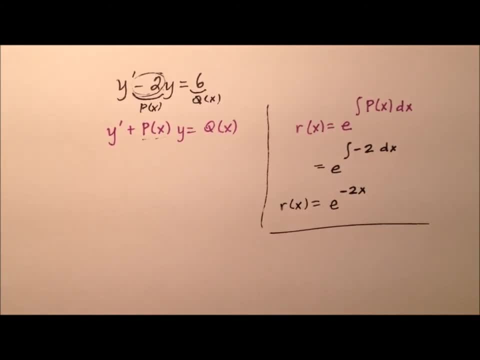 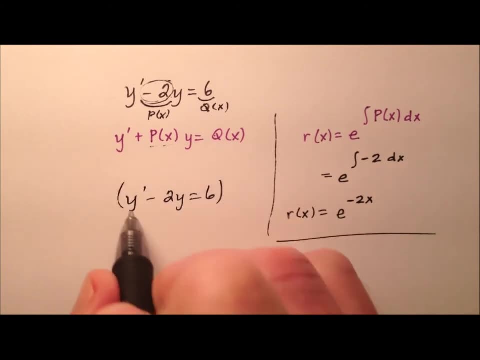 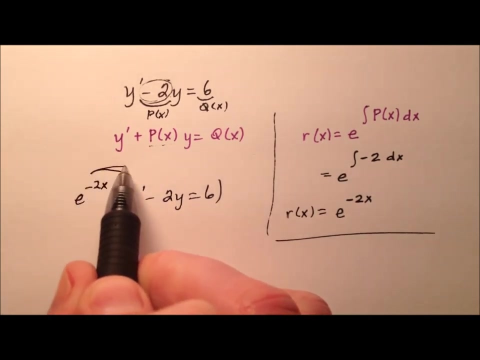 to equal e to the negative 2x. Well, what is it that we're going to do with that? Well, we're going to take our differential equation and we're going to multiply through by this integrating factor. I'm going to show you here in a second why we would do that. So every single term here is going: 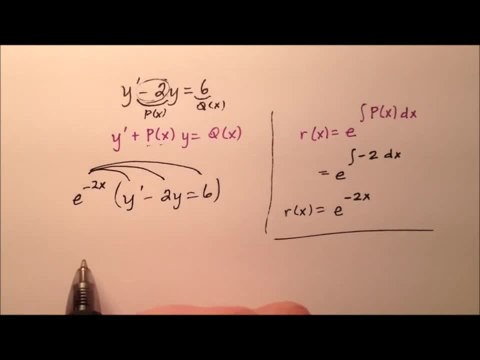 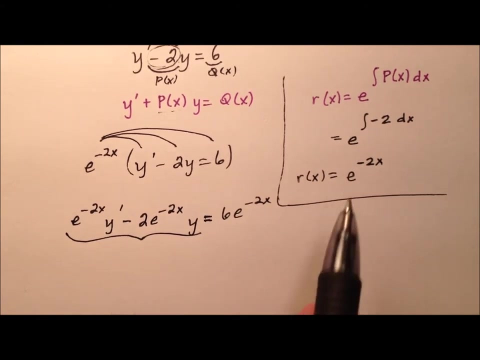 to get multiplied by this e to the negative 2x. So my equation now looks like: e to the negative 2xy, prime minus 2 e to the negative 2xy equals 6. e to the negative 2x On this left side. this is going to be really important and the reason we use this integrating 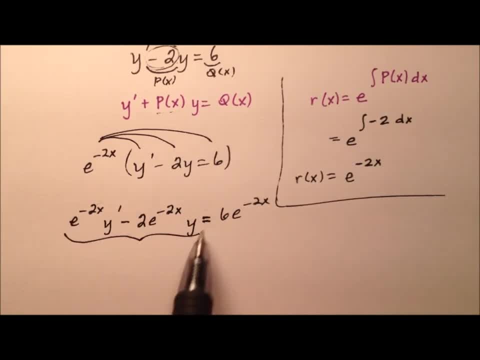 factor is because we kind of have the product rule going on here. So we have the function e to the negative 2x and you'll notice its derivative is negative 2, e to the negative 2x, and then we have y with its derivative y prime. So you can see this is in the form of the product rule. So to integrate, 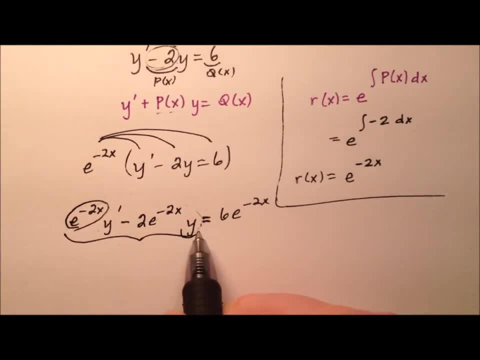 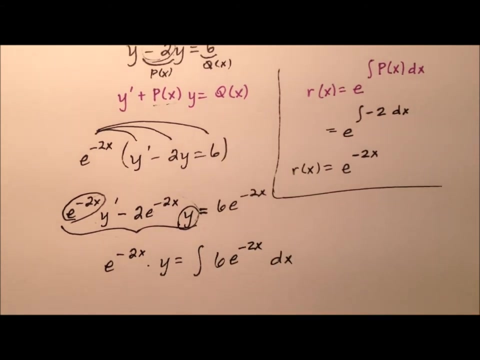 this would just be this function along with our y, So we can write e to the negative 2x times y and that will equal then the integral of our right side, 6 e to the negative 2x dx. Okay, so to take this integral, we can go ahead and use a little. 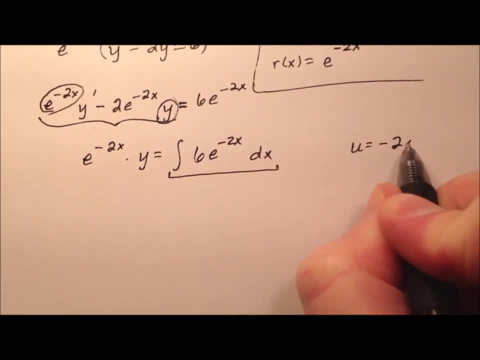 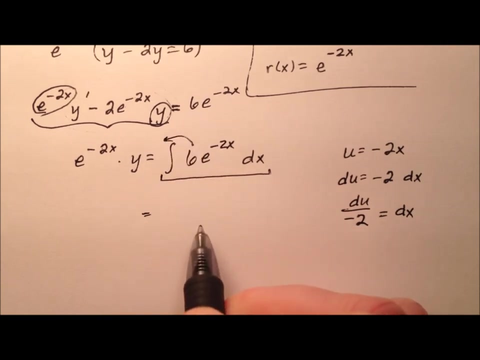 quick? u substitution if you would like, and we can just use negative 2x. So du equals negative 2x And then dx will be du over negative 2.. So the 6 you could bring out front if you wanted to, as a constant. So this would be e to the? u times du over negative 2, which of course could cancel. 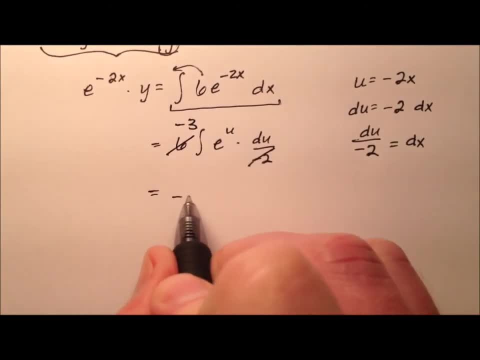 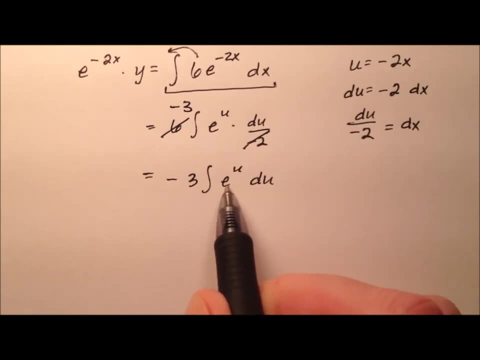 here and make this a negative 3.. So we have negative 3 times the integral of e to the u du, which of course the integral of e to the u is just e to the u. so we'll have our negative 3 e to the u. 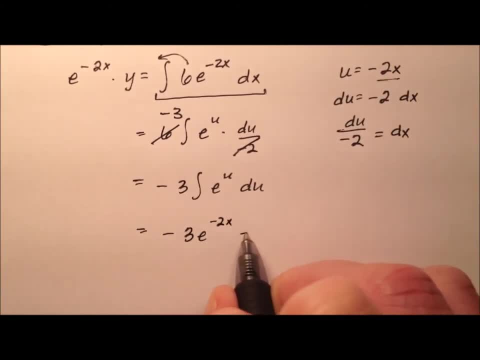 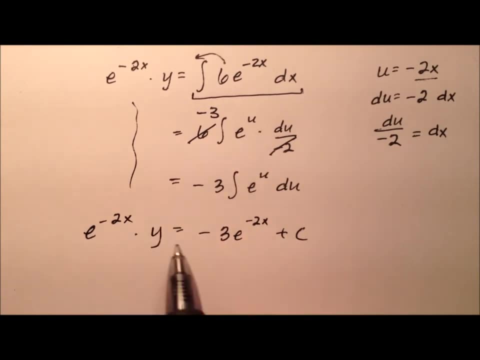 And u was negative 2 x, so go ahead and slip that back in Plus c. And then, of course, this left side came all the way down: E to the negative x times y. Okay, so we have integrated both sides of our equation. 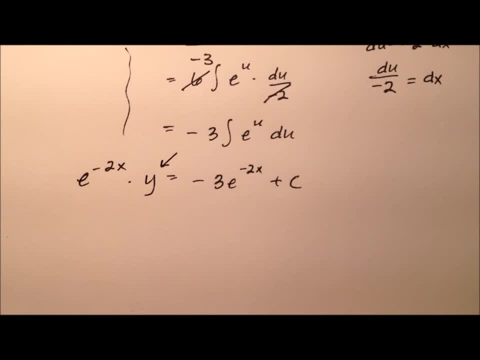 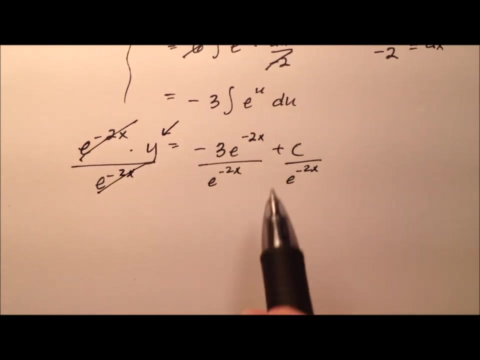 and this is what we're left with. So we'd like to solve for y here. to put it in explicit form, we're going to divide everything by e to the negative 2x On the left side. notice the e to the negative 2x is just cancelled, and also we have the term right. 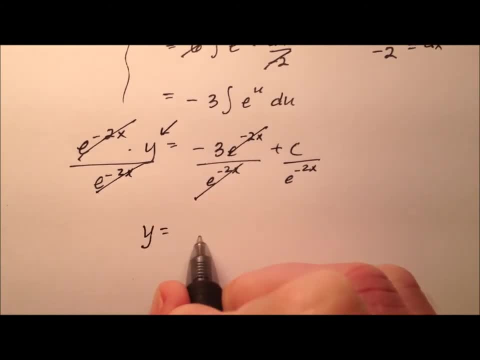 here where it does the same. So y will equal negative 3 plus in the denominator. here we kind of have the negative exponent, so we'll move it to the numerator to write it as a positive exponent. So here will be the solution of this first example, The first-order linear differential. 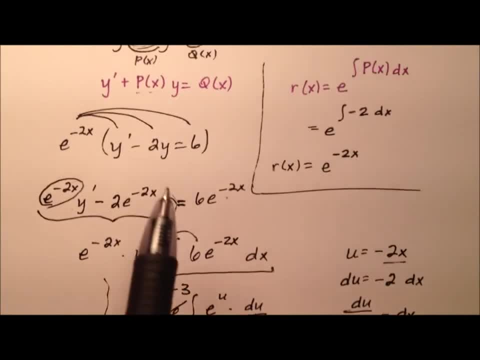 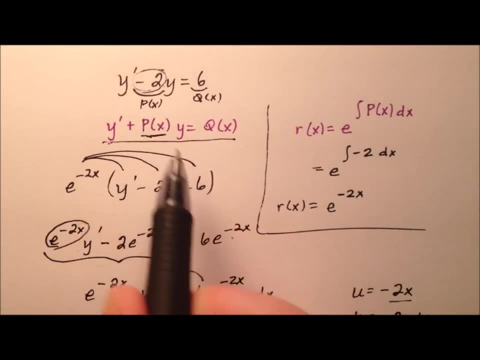 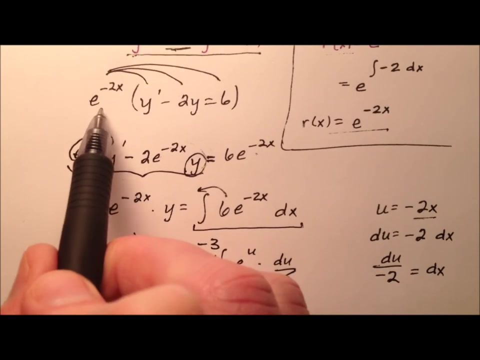 equation And the way we went ahead and did that recall was that we had to make sure that it was in linear form. then we grab the function p of x, which I included in the integrating factor. I multiplied the entire equation by that integrating factor. 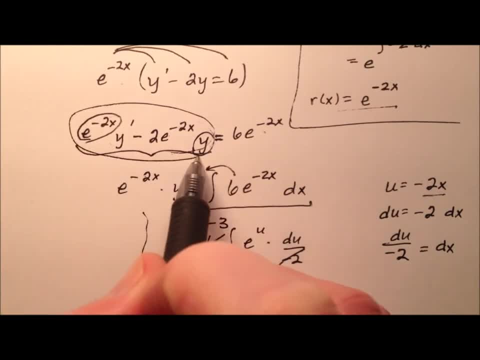 and the reason we do that is because it makes this letter less accurate. If we're going to do the whole equation that we into the linear form, which I included in the integrating factor, I multiply the entire equation by that integrating side of the equation into the product rule. So when I integrate that, it's 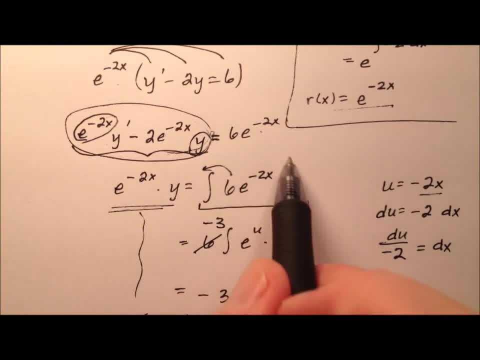 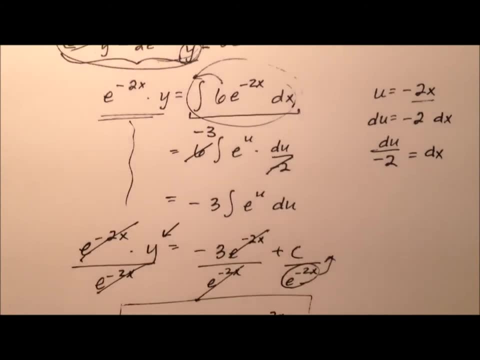 actually quite easy, And then I just have to worry about integrating the right side by itself. So, whatever rules you have to use, use substitution, integration by parts, whatever, And then I'm going to work through and solve for y In this. 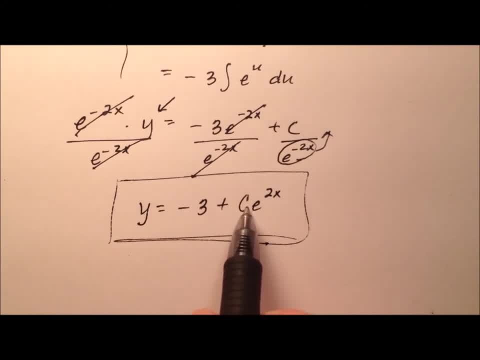 case I was not given an initial condition, so I was not able to find a particular solution, So I just had to leave it as a general solution, with my C right there. So that's the first example. So here in the second example that I'd 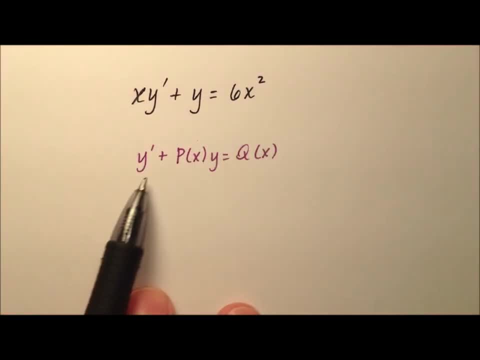 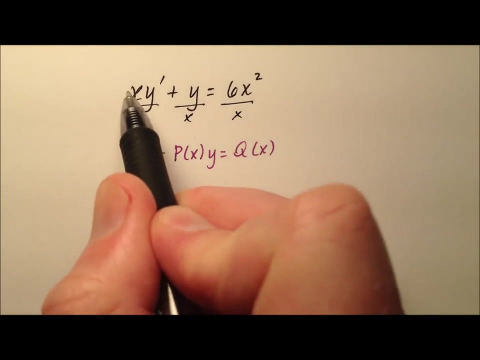 like to present to you our differential equation is not quite written in linear form, but we do see that it is first-order, because the highest derivative is the first derivative. So in order to get this y prime by itself, I'm going to go ahead and divide every term by X to begin with, And so the X's there. 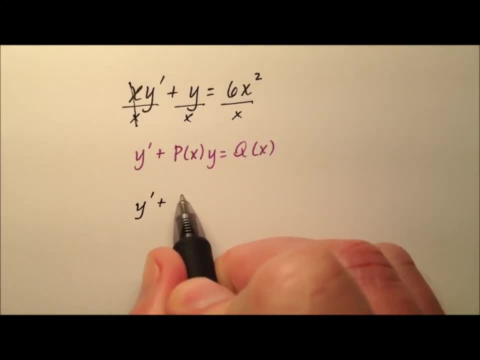 do cancel. So I have y prime plus one over E. So that's the first example. So in order to get this y prime by itself, I'm going to go ahead and divide every term by X to begin with, And so the X's there do cancel. So I have y prime plus one over. 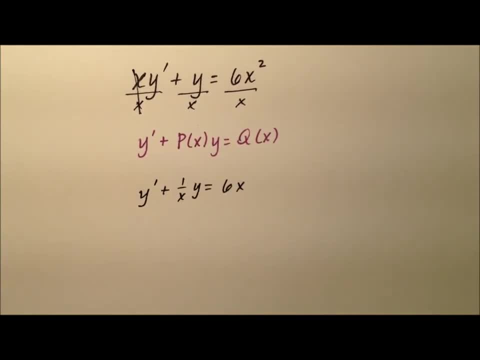 x, y equals 6x. Okay, so now it's written in linear form and of course, our p of x function is this: 1 over x, which is being multiplied by the y, and then our q of x is going to be just this 6x. 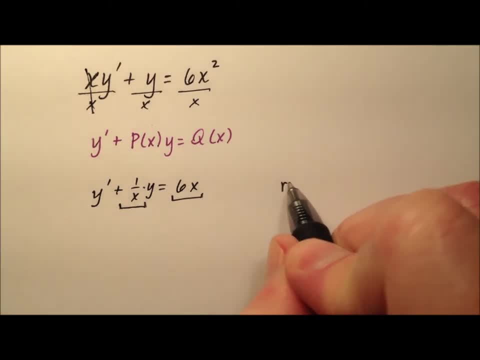 Okay, so the first big thing I have to do is go ahead and determine what my integrating factor is. So r of x equals e to the power of the integral of p of x, which is 1 over x, dx. and this integral, right there, is pretty straightforward. The integral of 1 over x with respect to x is just: 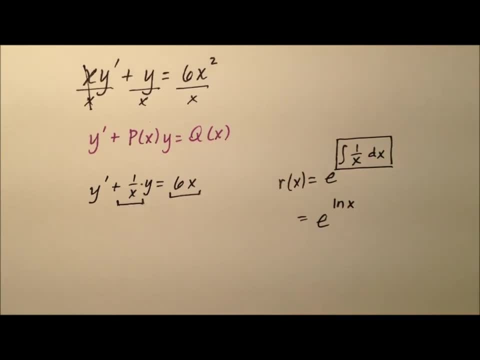 the ln of x. So I'm going to write it this way. and this is also nice, because we have e to the power of a natural log. So those are inverses of one another. So what we're left with for our integrating factor is the integral of p of x, which is 1 over x- dx. So we're going to write it this way. 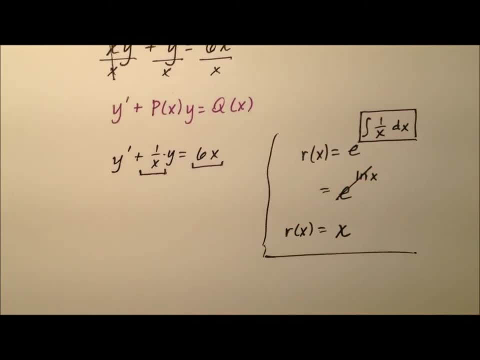 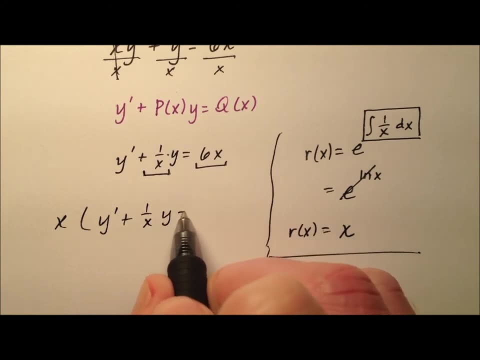 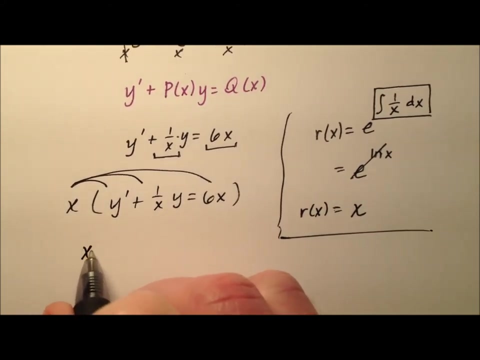 factor is just x. So we're going to go ahead, we're going to take our equation and we're going to multiply it through by x, So that x will be distributed to every term. So I have xy prime plus, and then x times 1 over x is just 1.. So it'll just be y and that'll be 6x squared. 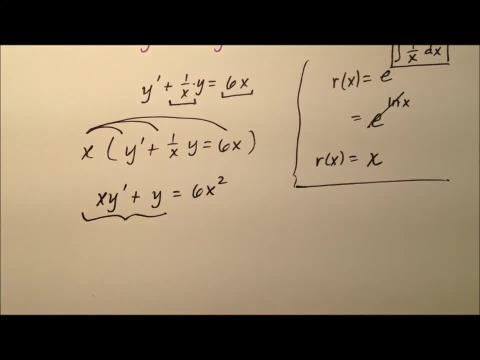 Well, as we talked about in the previous example, we do this integrating factor because it causes the left side of this to be a derivative, using the product rule. So when we need to integrate both sides, we have x, which is our function, and y, which is our function, and then the derivative. 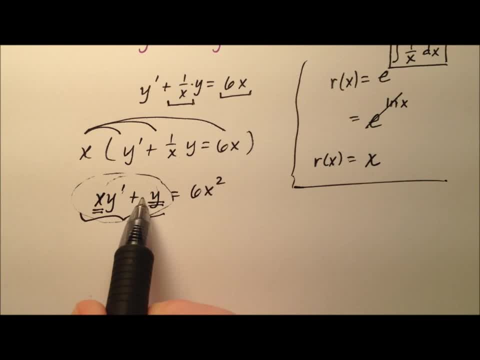 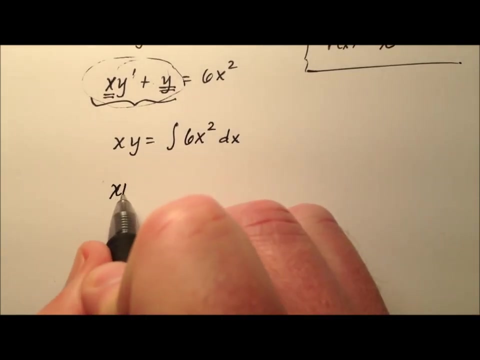 of y is our y prime and the derivative of x is 1.. So we're actually just going to write: xy equals, and then it's the integral of the right side, so 6x squared with respect to x. Okay, well, this is a pretty straightforward integral, So I'll have 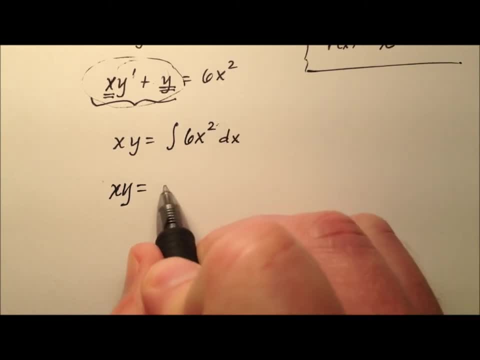 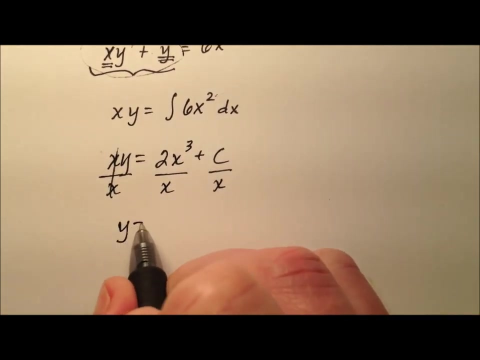 xy equals. we'll add 1 to the power, so 3, and then divide by that, So 2x cubed plus c is that integral. So to get y all by itself we can divide everything by x, so those cancel And y, it looks. 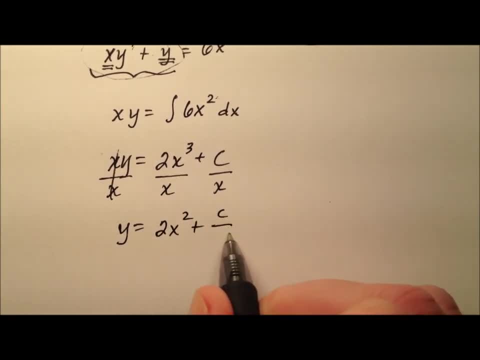 like is going to equal 2x squared plus x squared. So we're going to divide everything by x, and then we'll add y squared plus c over x, And here, once again, is a general solution, because I was not given.